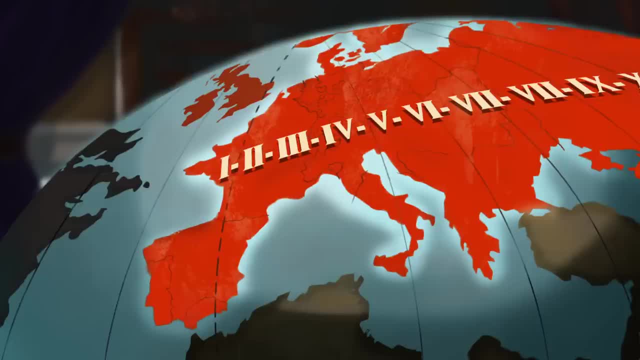 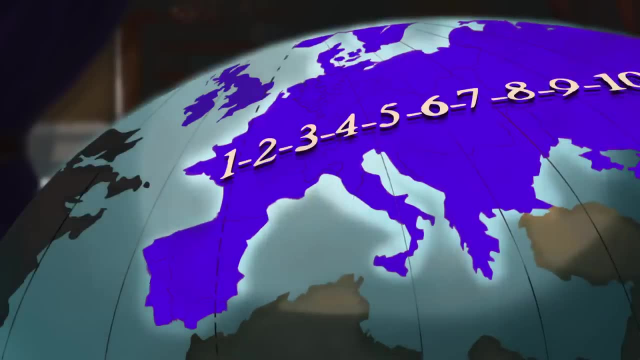 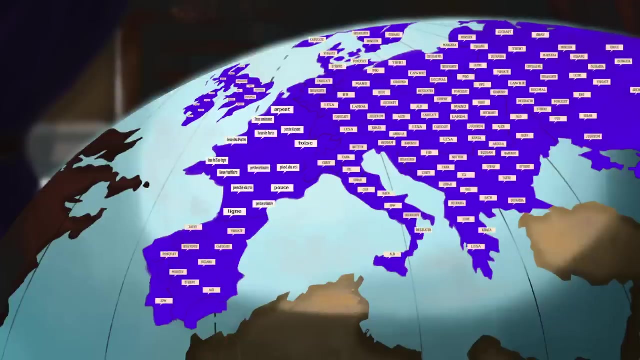 they had completely different number systems as well. By the late Middle Ages the Hindu-Arabic decimal system mostly replaced Roman numerals and fractions in Europe, But efforts by scholars like John Wilkins to promote standard decimal-based measures were less successful With a quarter. 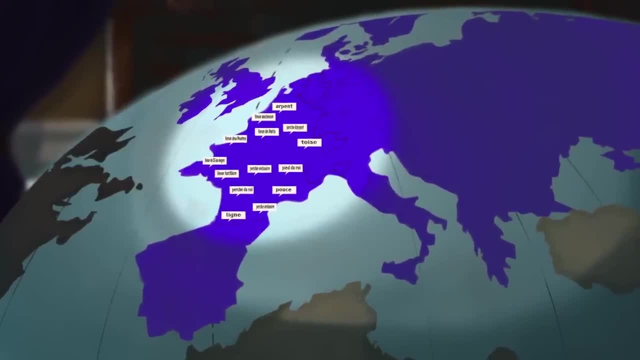 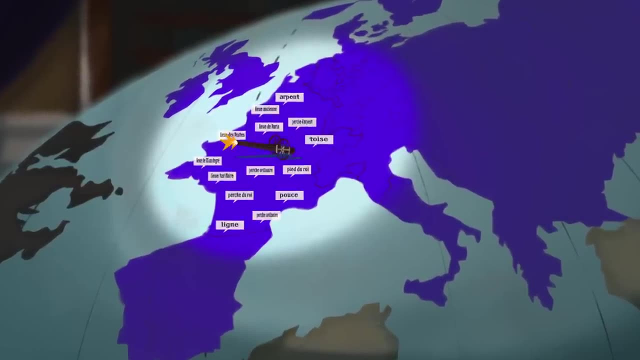 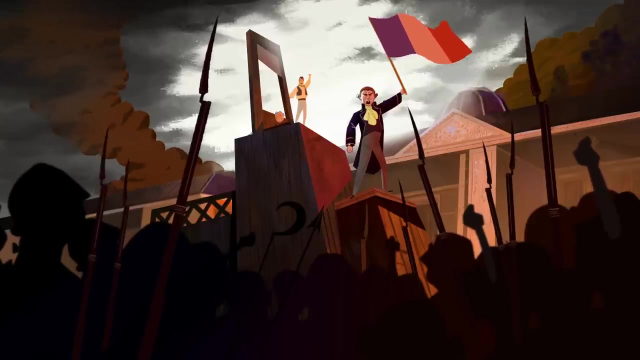 million different units in France alone. any widespread change would require massive disruption. And in 1789, that disruption came. The leaders of the French Revolution didn't just overthrow the monarchy. They sought to completely transform society according to the rational principles of the Enlightenment. When the new government took power, 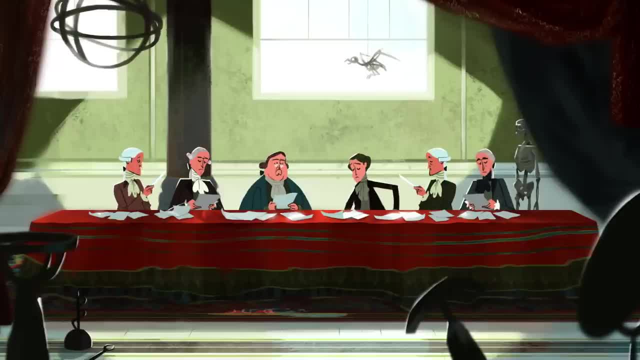 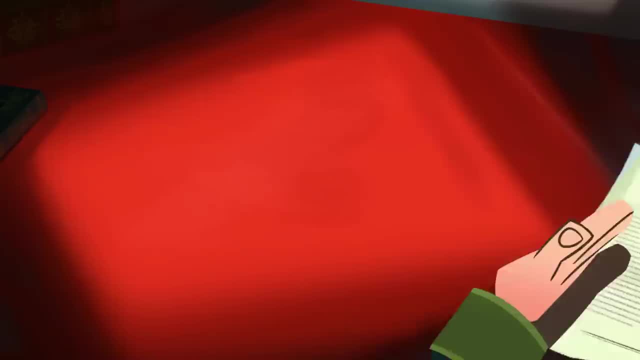 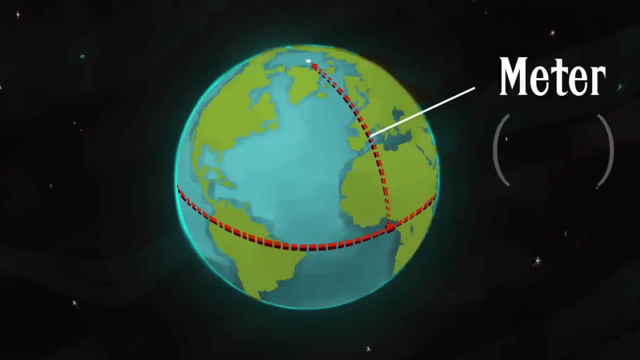 the Academy of Sciences convened to reform the system of measurements. Old standards based on arbitrary authority or local traditions were replaced with mathematical and natural relationships. For example, the meter, from the Greek word for measure, was defined as one ten millionth between the equator and North Pole, And the new metric system was in the words of the. 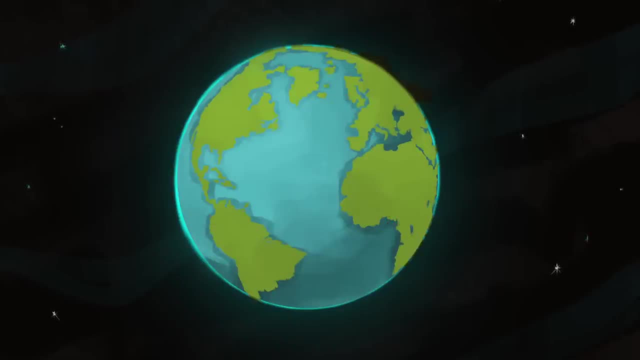 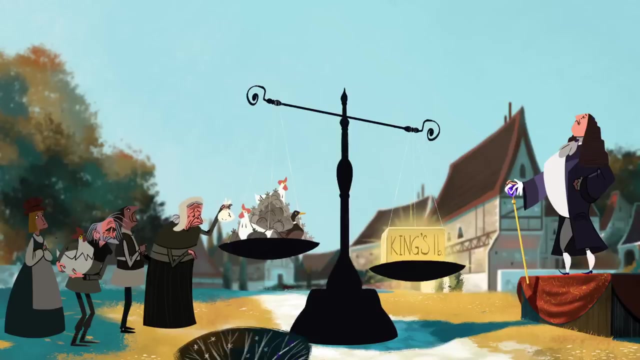 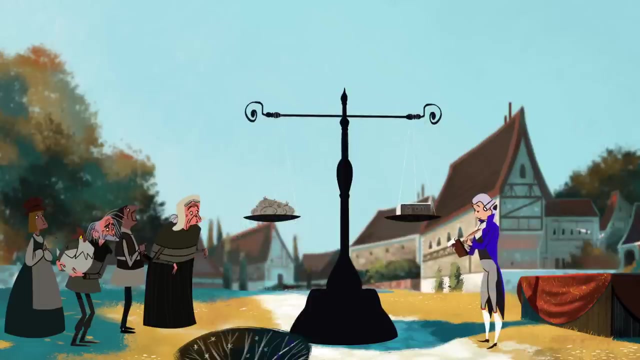 Marquis de Condorcet for all people, for all time. Standardizing measurements had political advantages for the revolutionaries as well. Nobles could no longer manipulate local units to extract more rent from commoners, while the government could collect taxes more efficiently. And switching to a new Republican calendar with 10 day, 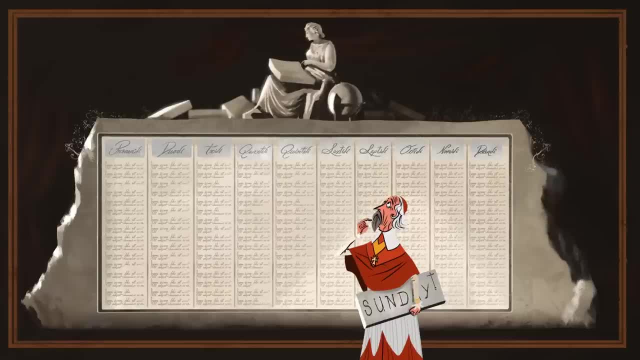 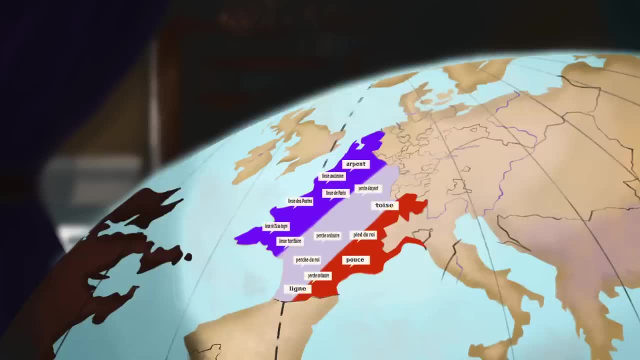 weeks. reduced church power by eliminating Sundays. Adoption of this new system wasn't easy. In fact it was a bit of a mess At first. people used new units to search but in reality they had not been able to spend more money to buy or sell a thousand tonne of money in one day. The levels of 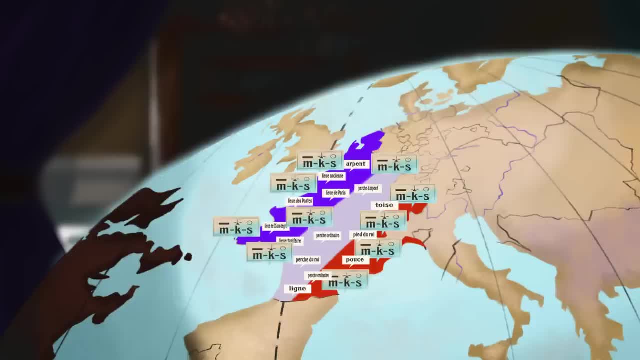 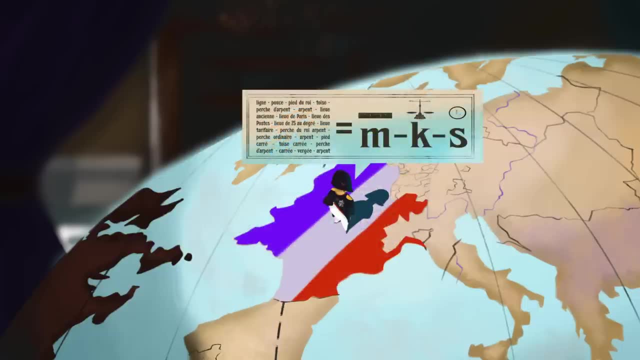 It used new units alongside old ones, and the Republican calendar was eventually abandoned. When Napoleon Bonaparte took power, he allowed small businesses to use traditional measurements redefined in metric terms, But the metric system remained standard for formal use and it spread across the continent along with France's borders. 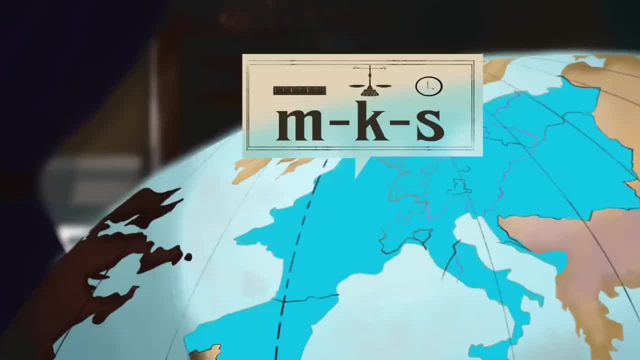 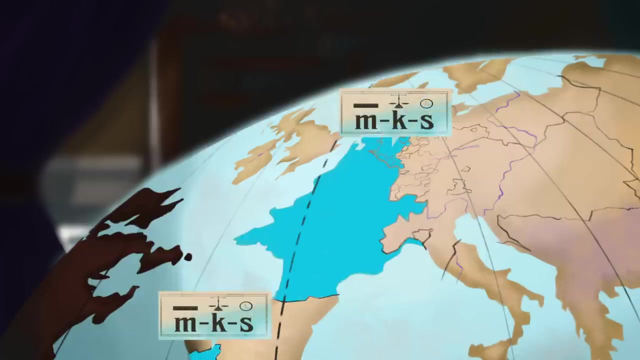 While Napoleon's empire lasted eight years, its legacy endured far longer. Some European countries reverted to old measurements upon independence. Others realized the value of standardization in an age of international trade. After Portugal and the Netherlands switched to metric voluntarily, other nations followed. 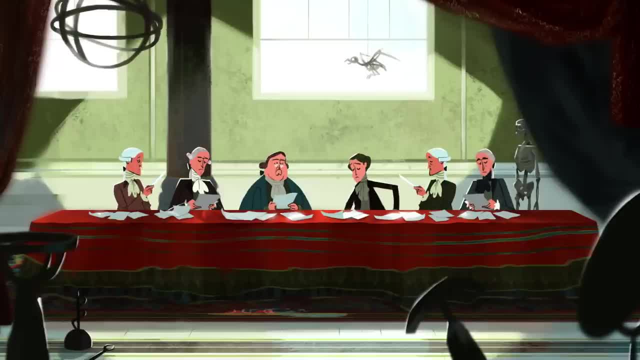 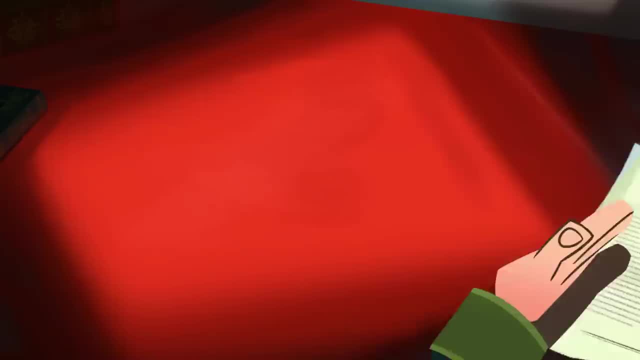 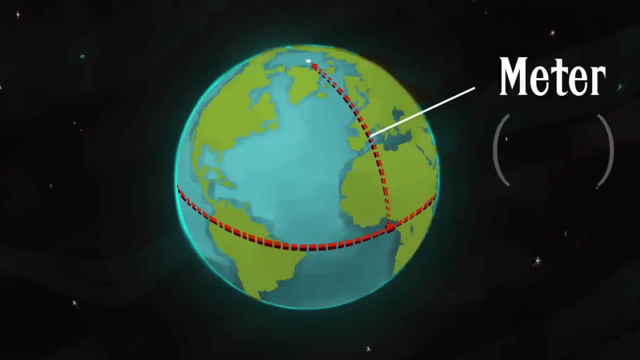 the Academy of Sciences convened to reform the system of measurements. Old standards based on arbitrary authority or local traditions were replaced with mathematical and natural relationships. For example, the meter, from the Greek word for measure, was defined as one ten millionth between the equator and North Pole, And the new metric system was in the words of the. 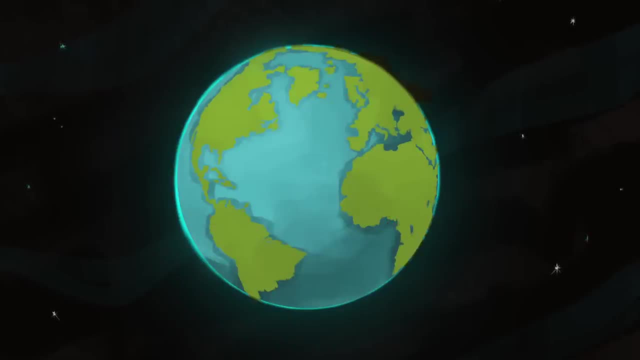 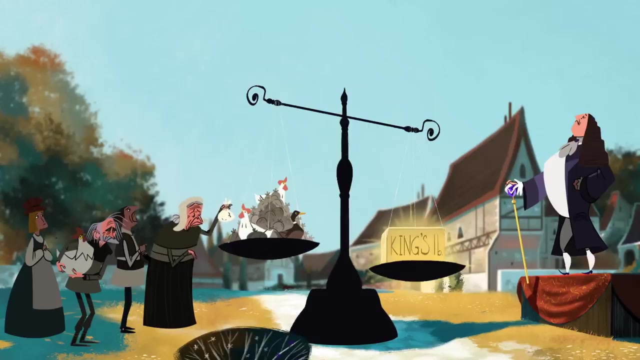 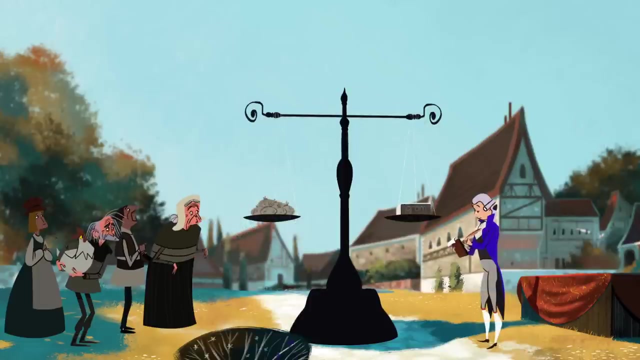 Marquis de Condorcet for all people, for all time. Standardizing measurements had political advantages for the revolutionaries as well. Nobles could no longer manipulate local units to extract more rent from commoners, while the government could collect taxes more efficiently And, switching to a new republican calendar with ten-day weeks reduced. 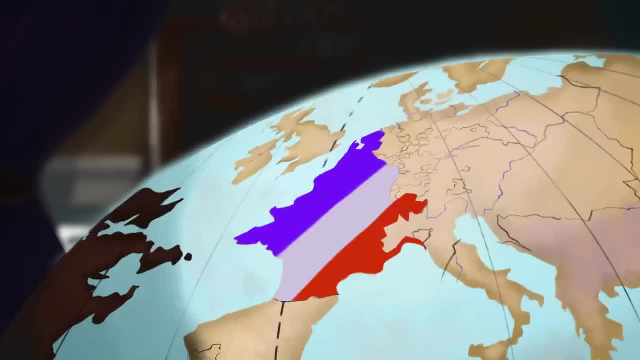 church power by eliminating Sundays. Adoption of this new system wasn't easy. In fact, it was a bit of a mess At first. people used new units to store their money, but then they stopped using the new system, And that's why the new system was so difficult to adopt. The new system was more efficient and more efficient than the old system. The new system has now been replaced with a new system With a greater number of new units. the system was slowly becoming more and more complex, But the new system was more and more complex. The new system was more and more complex. The new system was more and more complex. The 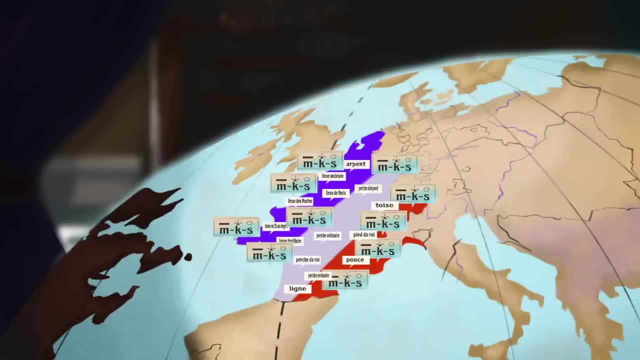 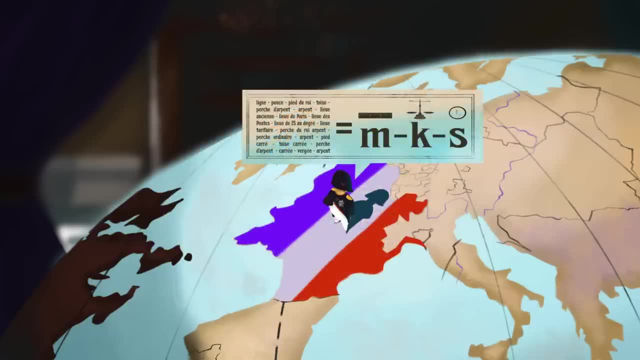 First, people used new units alongside old ones, and the Republican calendar was eventually abandoned. When Napoleon Bonaparte took power, he allowed small businesses to use traditional measurements redefined in metric terms, But the metric system remained standard for formal use. 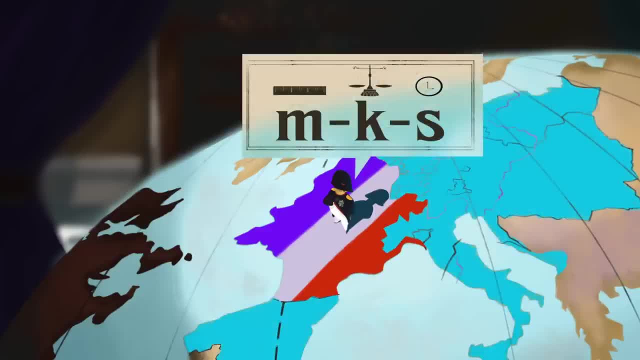 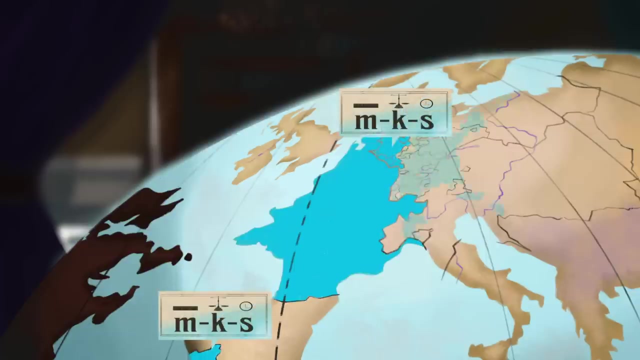 and it spread across the continent along with France's borders. While Napoleon's empire lasted eight years, its legacy endured far longer. Some European countries reverted to old measurements upon independence. Others realized the value of standardization in an age of international trade After Portugal and the Netherlands switched to metric voluntarily. 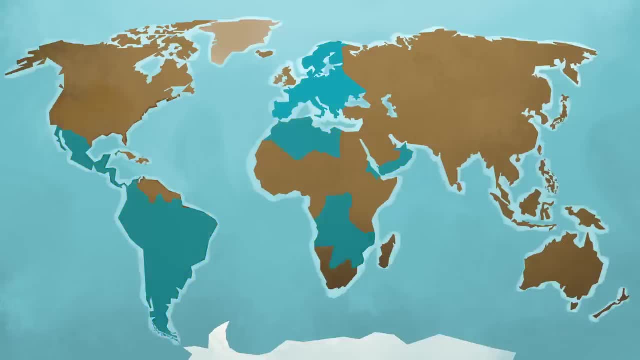 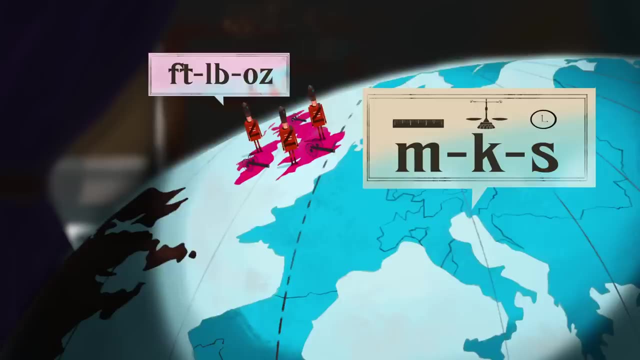 other nations, followed with colonial empires spreading the system around the world. As France's main rival, Britain had resisted revolutionary ideas and retained its traditional units. But over the next two centuries, the British Empire slowly transitioned, first approving the metric system as an optional alternative. 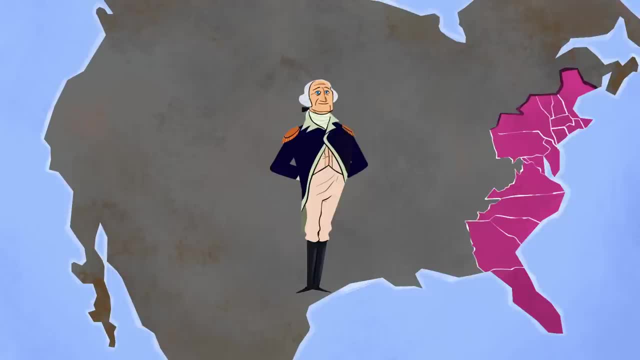 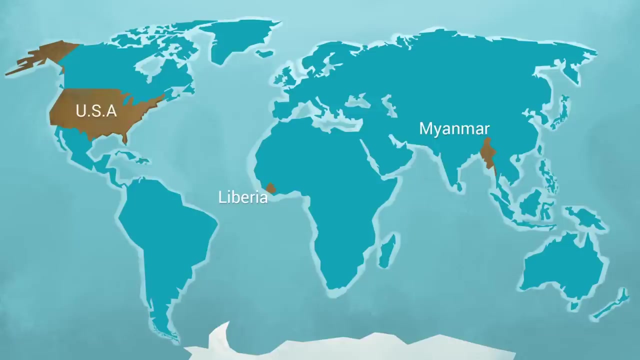 before gradually making it official. However, this switch came too late for 13 former colonies that had already gained independence. The United States of America stuck with the English units of its colonial past and today remains one of only three countries which haven't fully embraced the metric system.